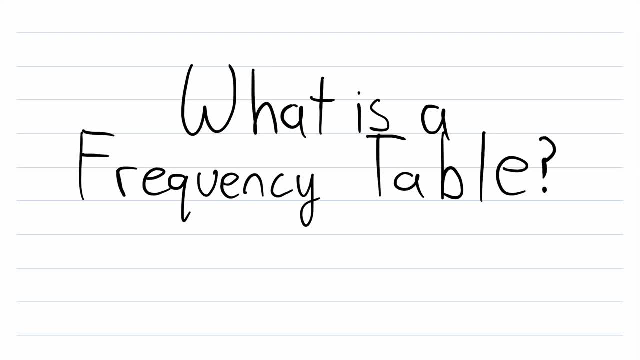 Hey everyone, welcome back to Wrath of Math. In today's video, we'll be answering the question: what is a frequency table? There are a lot of ways to organize data, and frequency tables are just another one of those ways. So let's look at some data and create a frequency table for it to learn. 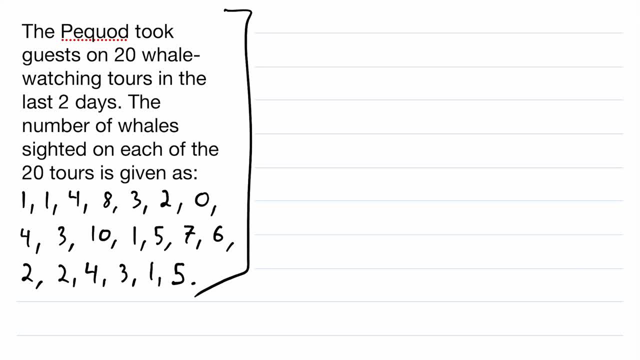 more about what exactly they are. Alright, so here is our situation and some data. The Pequod, which is a ship, took guests on 20 whale watching tours in the last two days. The number of whales sighted on each of the 20 tours is given as, and then our data is listed. So each one of these. 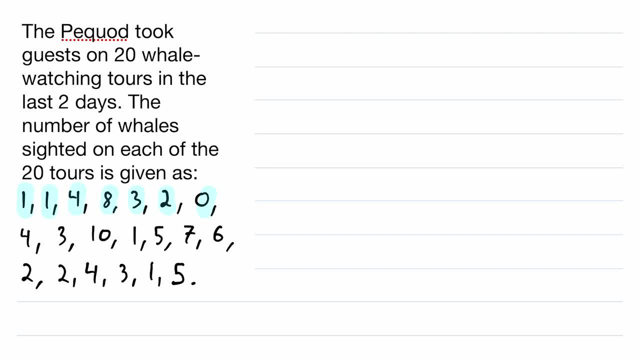 numbers is the number of whales seen on one of 20 whale watching tours. So let's go ahead and make a frequency table for this data, which will make it very easy to see how many times each data point occurred. A basic frequency table usually has two to three columns, and ours will be no different. 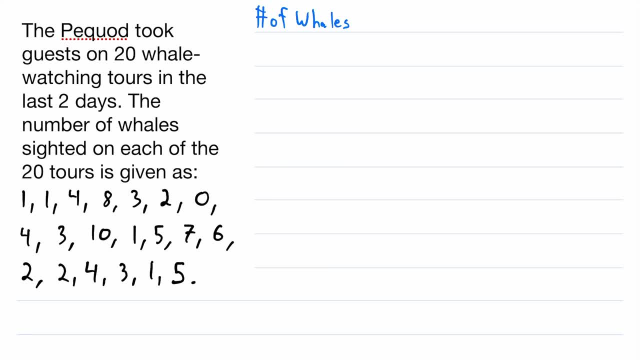 So in this first column- the number of whales- we'll be putting the distinct data points that we have in our data set, So there will be one row for each distinct data point. The second column is the tally column, and this column certainly isn't necessary, but it's going to help us count. 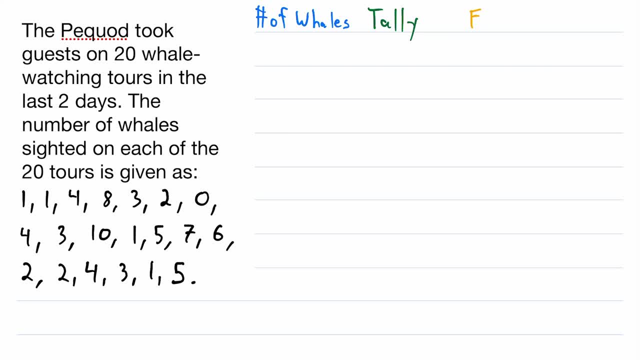 up the frequency of the different data points. The third column, of course, is the frequency column, which tells us how frequent each data point is, which is how many times each data point occurred in the data set. The tally column actually tells us the same information, but the frequency column 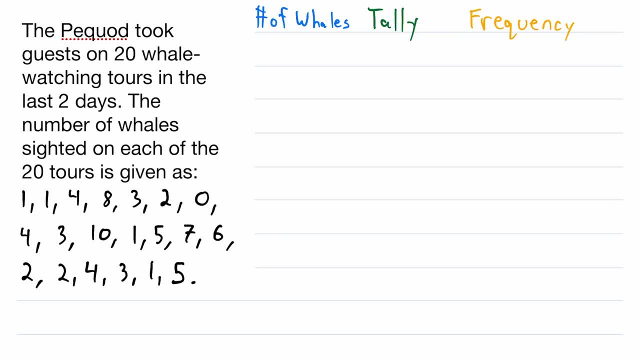 does it a little bit better. That should all make a bit more sense in a couple minutes. Now let's add some structure to this table. We wouldn't want to go on with an unorganized frequency table, so we'll add these nice straight. 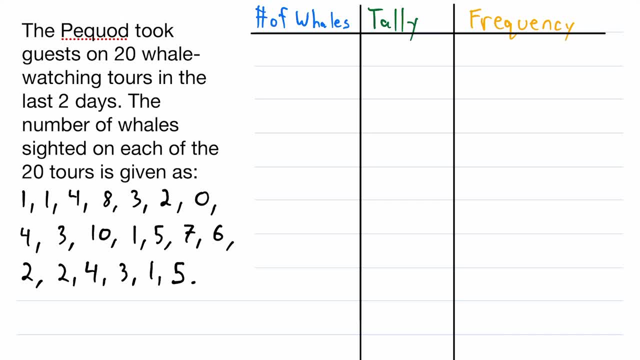 lines here and keep everything nice and organized. All right, so let's start making this table In the first column. like I said earlier, we'll have a row for each distinct data point. Looking over at our data set, I see that the distinct data points are 1,, 4,, 8,, 3,, 2,, 0,, 10,, 5,, 7, and 6.. 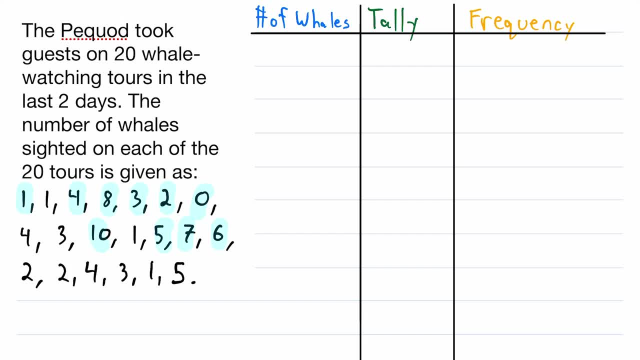 So every integer, from 0 to 10, or 9, is in our data set. So I'll start writing them here Again, a row for each distinct data point, and we're going to list them in order from least to greatest. Now I'm going to have to zoom. 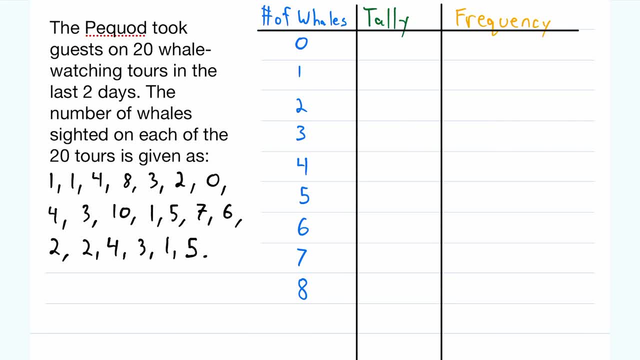 out a little bit so that we have room for every row on the screen. That should be just enough, All right. and then in the last row we put a 10.. So here we have one row for every distinct data point. So our first column is done. Now we move on to the tally column. We kind of use this column as 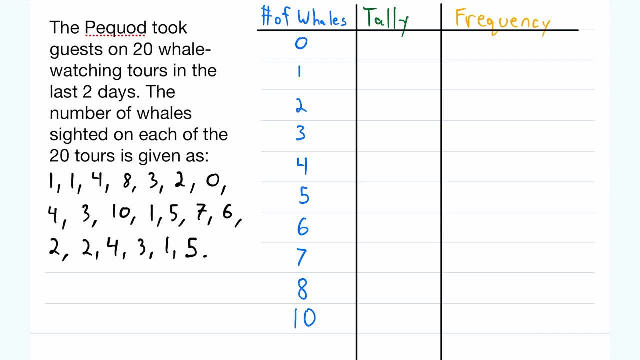 scratch work. All we're going to do is look through the data point by point and tally up the number of times we see each data point in this tally column. So let's get to it. First few points I see are 1, 1, and 4.. So I'll put two tallies in the one row and one tally in the four row. Then we 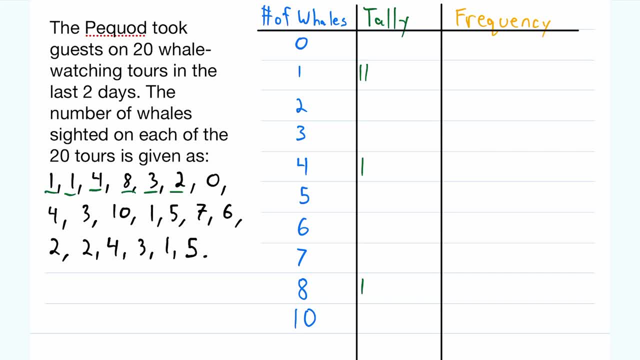 have 8,, 3, and 2.. So one tally on the 8 row, one on 3, and one on 2.. Then 0,, 4, and 3.. So a tally at 10,, 1,, 5.. So a tally for 10,, tally for 1,, tally for 5.. 7,, 6,, 2.. So I'll put a tally at 7,, tally at 6,. 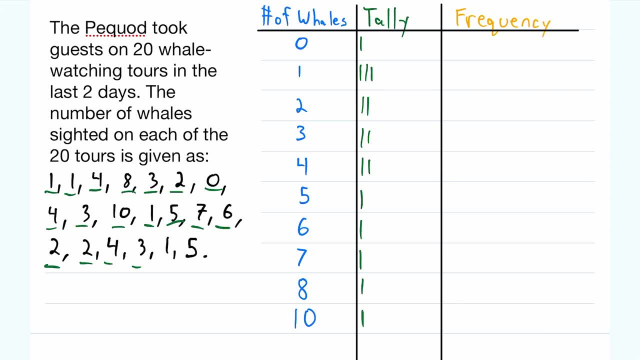 and another tally at 2.. Then 2,, 4,, 3.. So another tally at 2,, another tally at 4,, another tally at 3.. And then, finally, 1 and 5.. So another tally for 1, and another tally for 5.. Now for the frequency. 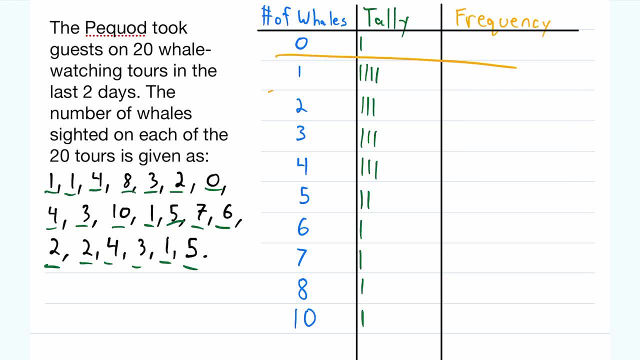 column. we just have to count up the number of tallies in each row and put that number in the respective row of the frequency column. So we see there was one whale watching tour that saw zero whales, so we'll put a 1 in the frequency column. There were four tours that saw one whale, so in 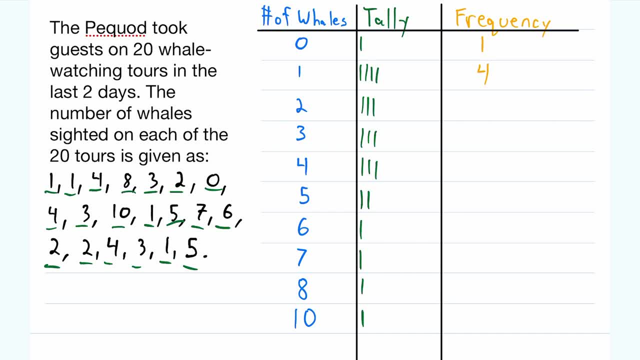 this row. we put a 4 for the frequency column And we continue in this way. This was a 3.. Three tallies here, three tallies here, two tallies here and then 1,, 1,, 1, and 1.. We just counted up the tallies. 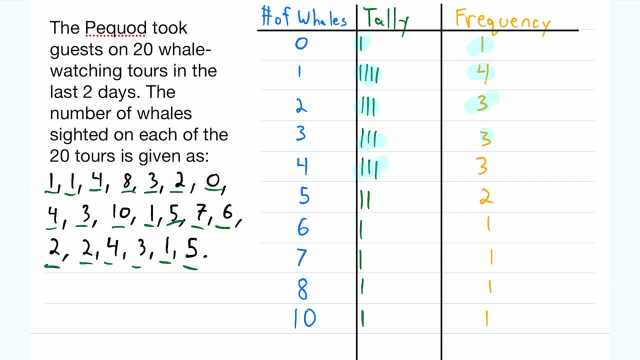 and converted each one to a numeral for the frequency column. So now we're done. This is a completed frequency table for this data set. Something you can do with a frequency table to make sure you didn't miss anything is add up all the numbers in the frequency column. They should. 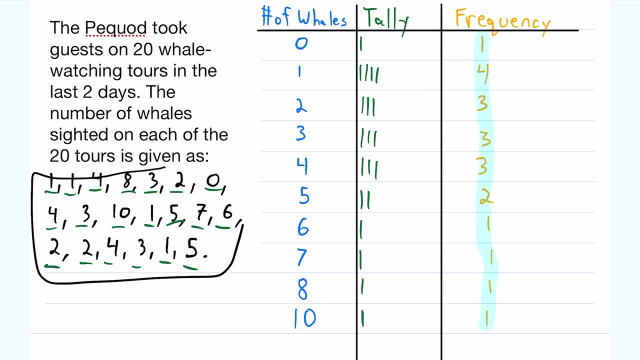 add to the total number of data points that you had in your data set. If they don't add to that, then you made a mistake somewhere. In this case, adding up all our numbers in the frequency column gives us 20, just like we want, because we had 20 data points Once you've created a frequency table. 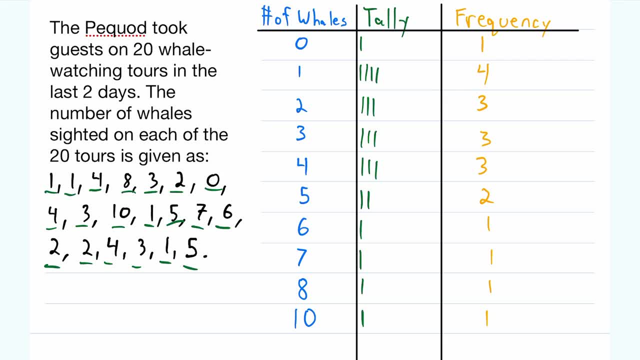 all that's really left is being able to read it and interpret it. So just remember that each row in the first column is a distinct data point that appeared in our data set and then in the frequency column we have the number of times that data point. 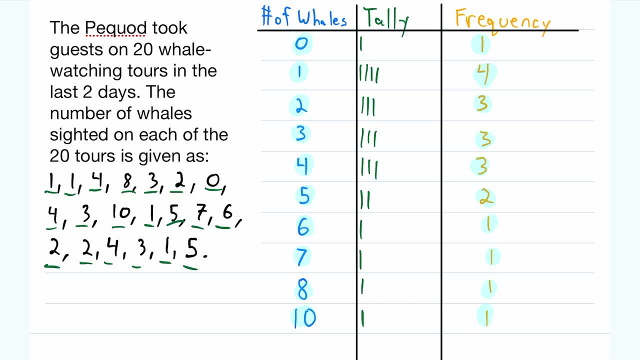 occurred and the tally column can pretty much be ignored at this point. It's really only helpful for us when we're creating the table. So let's just go over a little bit of information you could interpret from this frequency table If we add up the first four rows in this frequency column. 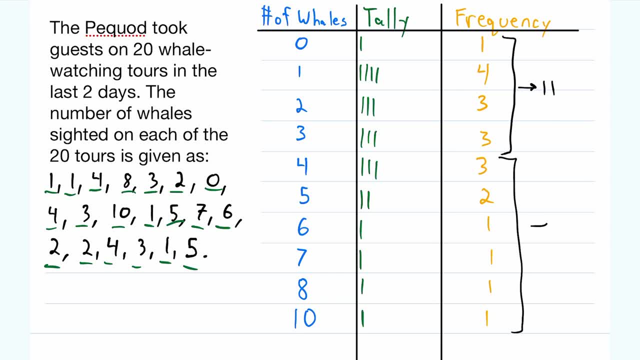 we get 11.. If we add up all the rows below that, we get 9.. 11 is just over half of the total number of data points, since we have 20 data points. So from this information we're able to conclude that just over half of the whale watching tours. saw three whales or fewer, and just under half of the whale watching tours saw four whales or more. Another thing you might notice if you were thinking about going on one of these tours is that 19 of 20 tours saw at least one whale, and that's pretty important. 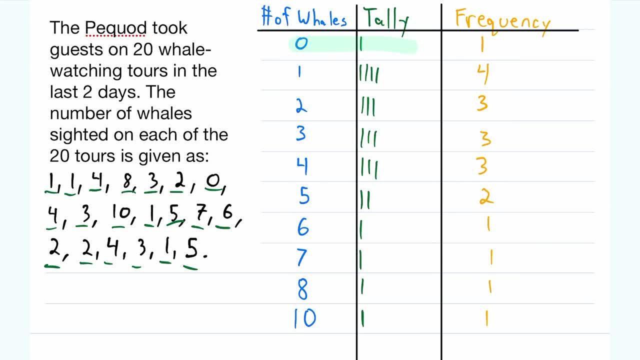 information, since the whole point is to see a whale. You can see that only one unlucky tour saw zero whales. You might also notice that the most whales any tour saw was 10, which only happened once. So there's a lot of information that we can get from this frequency. 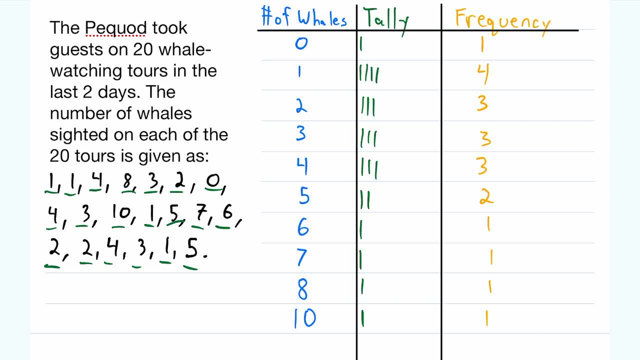 table and I want to issue a quick disclaimer that this data is made up, so I have no idea if this accurately represents the number of whales seen on your average whale watching tour, but I'd like to go on one soon and get a data point for myself. Anyways, this is what a frequency table. 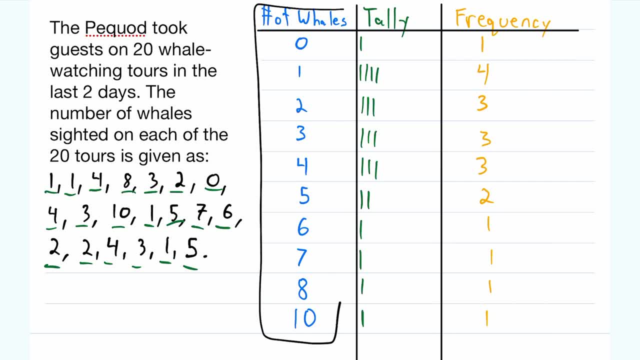 is, and that's how we make it. In the first column we put our distinct data points, We use the second column to tally up how many times each data point occurs while we look through our data set, And then in the frequency column, we just convert each tally to a numeral, so that it's nice.